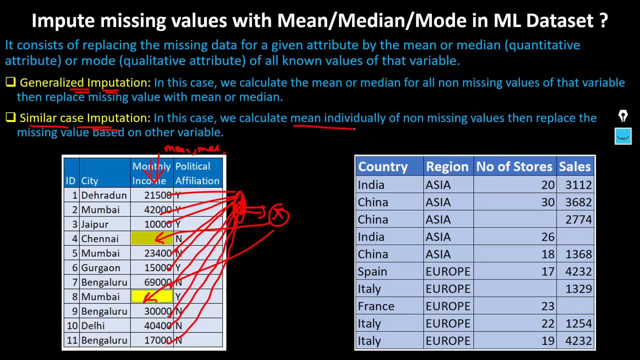 so in this case we calculate mean individually of non-missing value, then replace missing value based on other variable. it means what we will do here: this is your missing value, this is your missing value. so what we will do, we will calculate the mean individually. it means we will calculate. 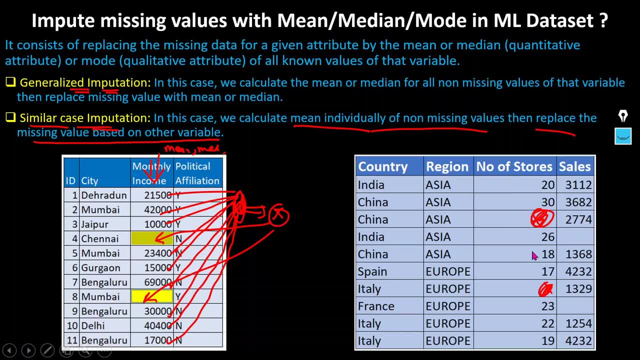 the mean individually. so what we will do, we will use the mean by using the other column. it means, as we can see, that these are the similar data. so what we will do, we will calculate the mean taking asia. so what we will do. so we will calculate the mean of the store which belong to the region asia. 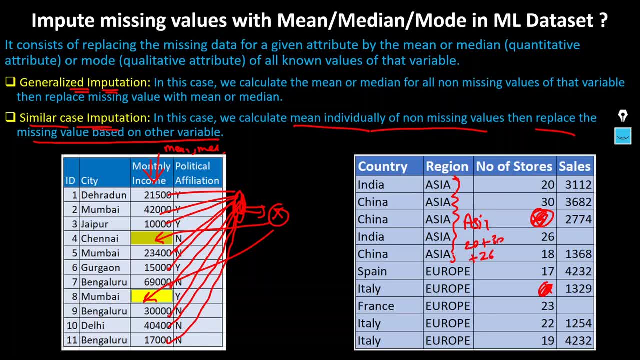 it means what we will do. we will take 20, 30, 26 and 18, then divided by 4.. so in this case, whatever the value we will get, we will impute at this place now again, what we will do. we will take the mean. 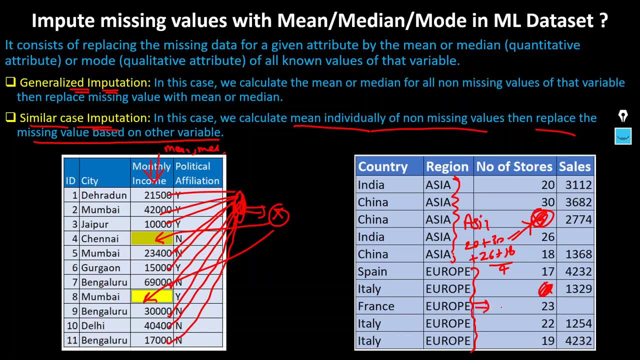 by using the europe data and we will, whatever the value we will get, we will impute here. it means we will consider only this data. these data we will only consider and after that, whatever the value we will get, we will use at this place. so this way we use mean and median by considering the other. 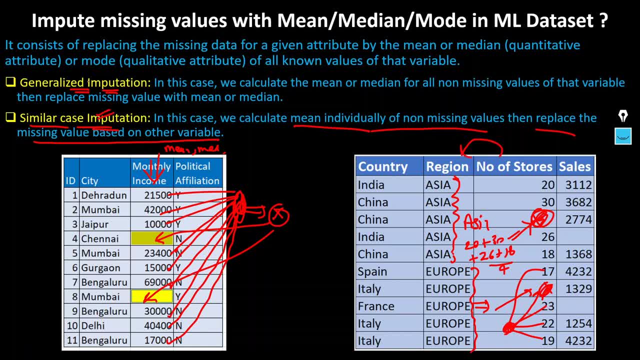 variable that is called as a similar case imputation and in generalized way we only use the mean. and in similar case imputation we impute x variable by considering the by variable. how we impute the missing value for the categorical variable. let, this is your categorical variable. 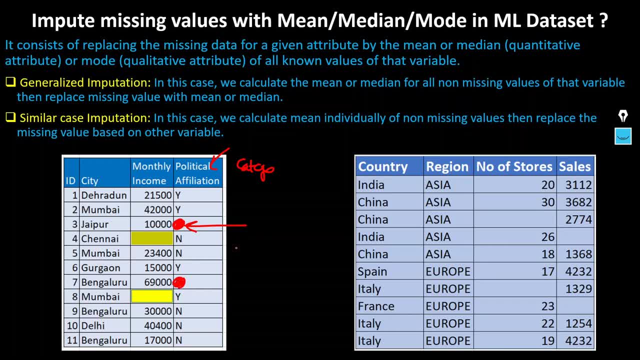 and these are the missing value. so what we will do, we will use mode mode of political affiliation: one, two, three, four, four. yes, one, two, three, four, five, five is no. so what we will do, we will use five because mode is five here. so we will impute n and n here, so this way we can impute the missing. 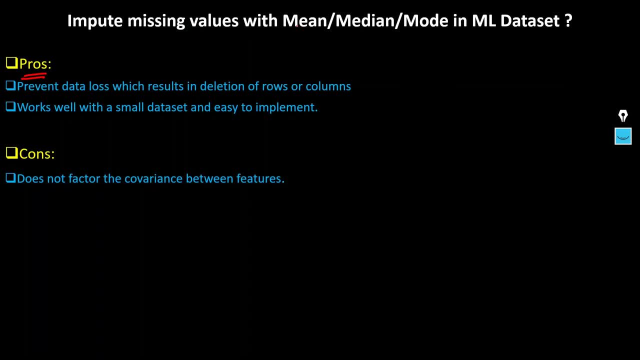 value for a categorical variable. what is the advantage of using the mean and median and mode? it prevent the data loss which result in deletion of the row and column, as we had discussed in our previous video, where we have deleted all the rows. that. this is your data frame. this is your